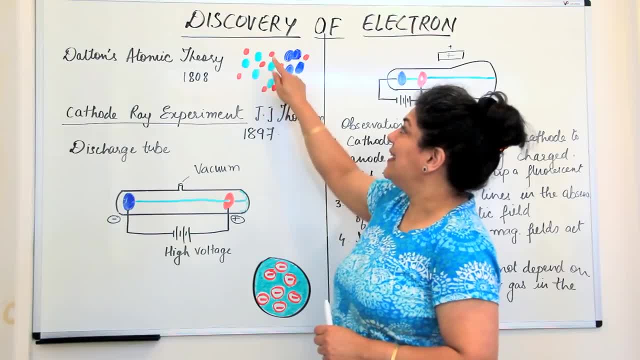 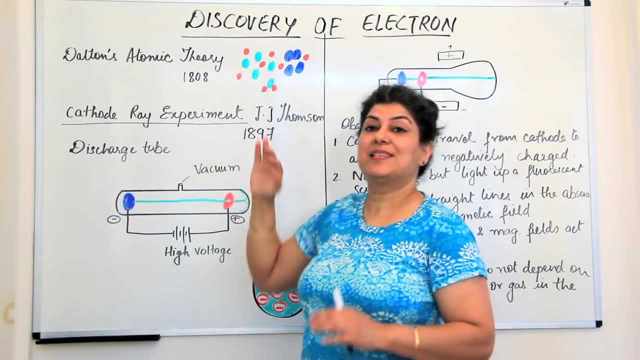 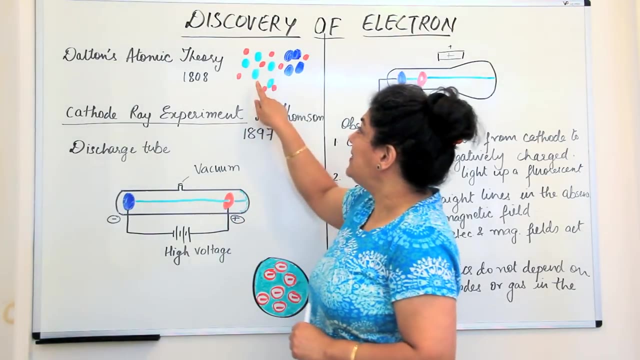 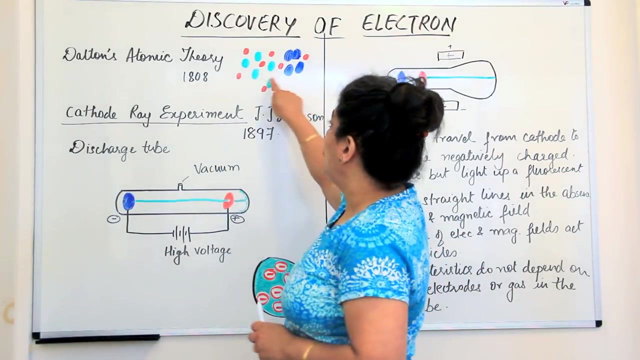 Dalton then gave his atomic theory, where he said that atoms are actually the smallest particles of matter and atoms of different elements are different from each other in their masses but atoms of the same element are identical, and that atoms of different elements, they combine together to form compounds Now, which today we know as compounds. But 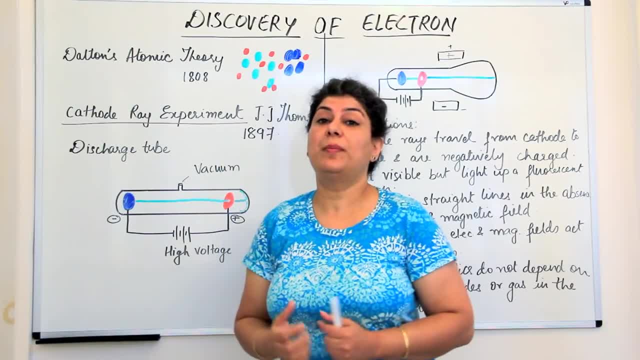 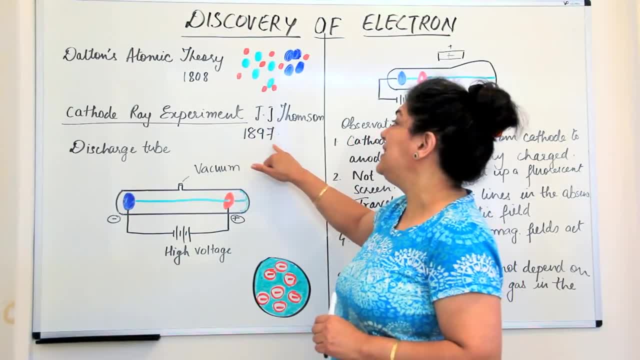 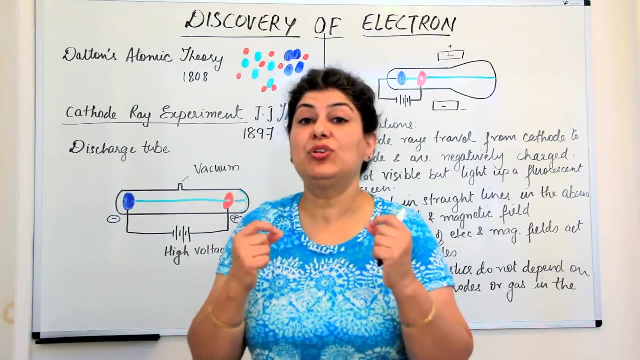 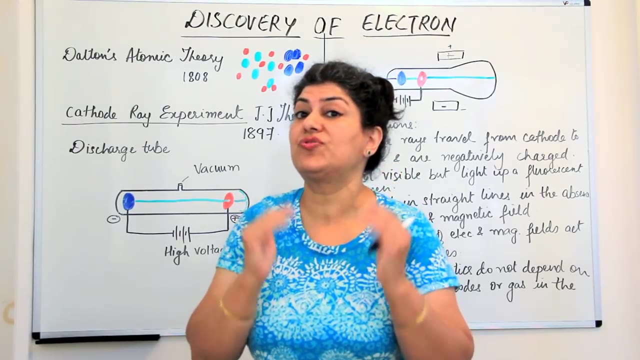 particles. At the end of the century in 1897, JJ Thompson and other scientists. they were working on atoms and they were trying to find out what atoms. they wanted to find out the properties and wanted to learn about atoms and wanted to know the. 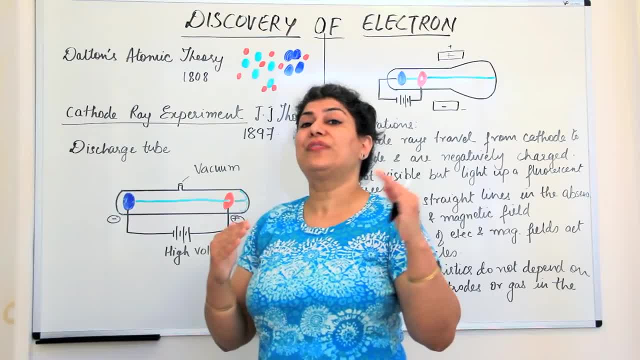 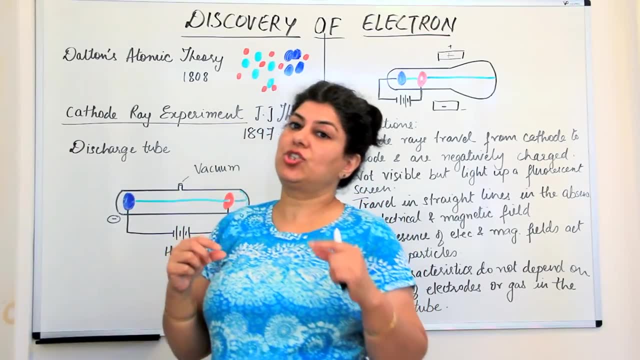 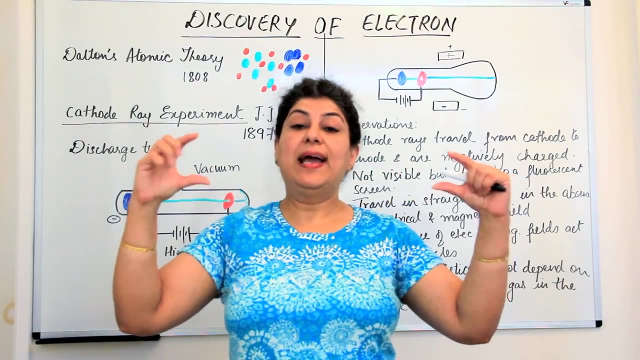 structure of an atom. So they were carrying out lots of experiments. Thompson carried out an experiment in a discharge tube. I would like you to imagine the discharge tube to be somewhat like a tube light that you have in your rooms. the tube light is a glass tube and it has 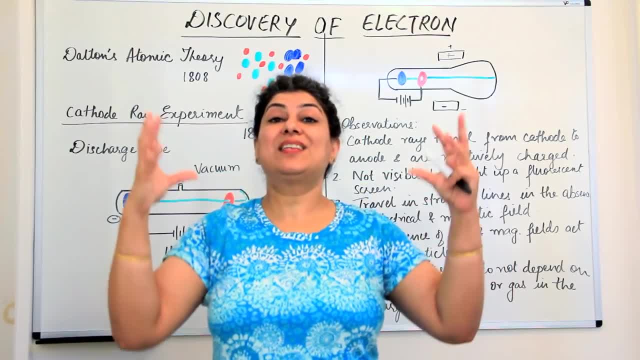 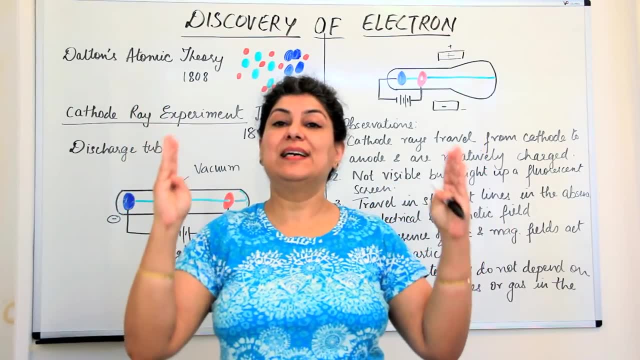 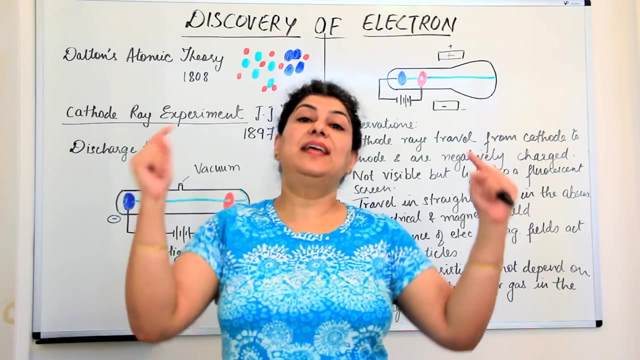 got a fluorescent coating on it which is, and when it lights up you can see the light. the fluorescent screen lights up and you see it, and the two ends of the tube light. they've got metallic what discs which are in the end and which are connected to the electric source and they produce the electricity and which 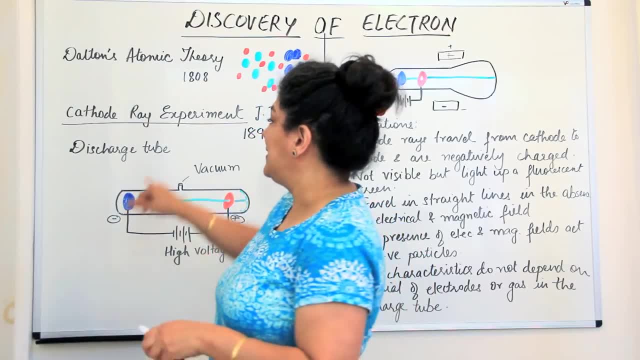 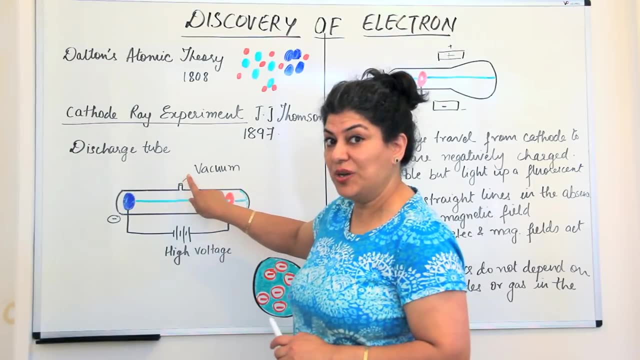 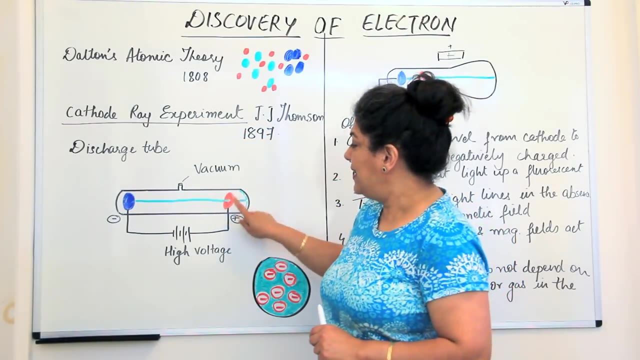 produces the beam of light and which illuminates the tube light. in the same way, he used this discharge tube, which was like a tube light and it had an opening here which was connected to the vacuum pop. so what did he do? That? he took a gas in this like hydrogen, and he connected. the two electrodes were called 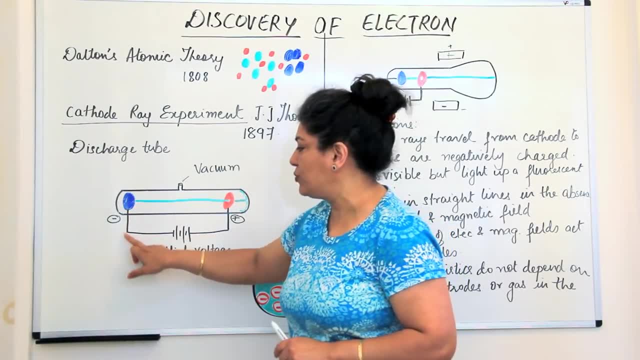 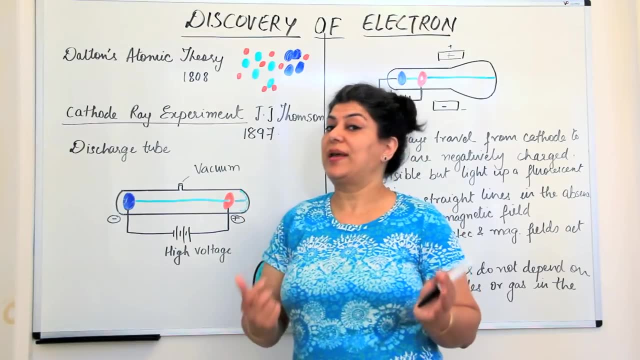 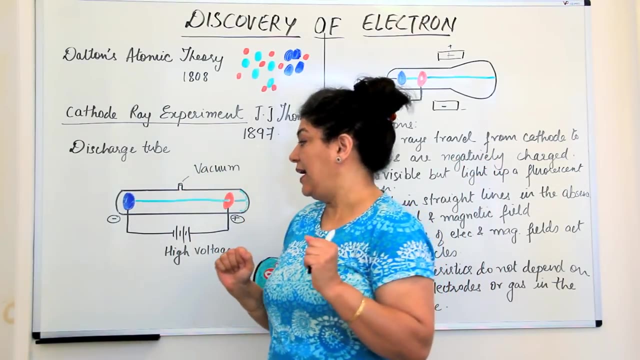 the cathode and the anode. this is called the cathode because it was connected to the negative terminal of the battery, of the source of electric current, and the positively charged electrode was known as the anode. what did he do when he took hydrogen? he passed electric current through the hydrogen at one atmospheric pressure and 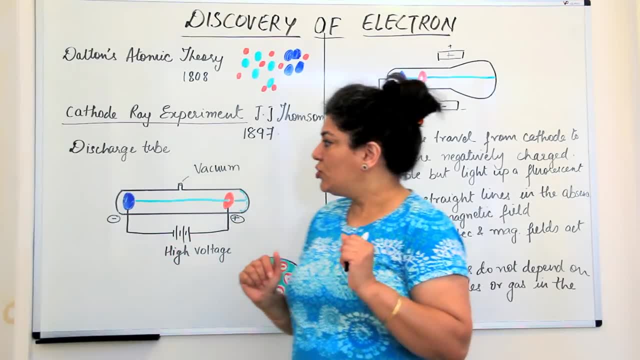 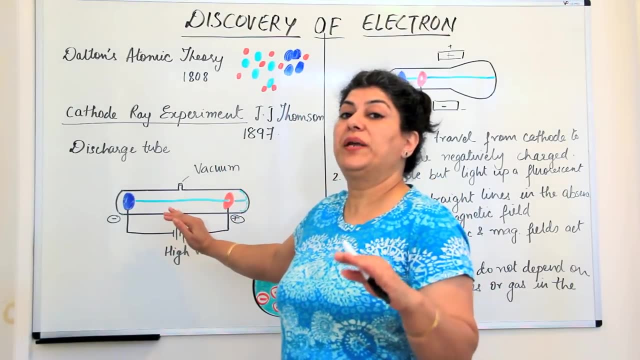 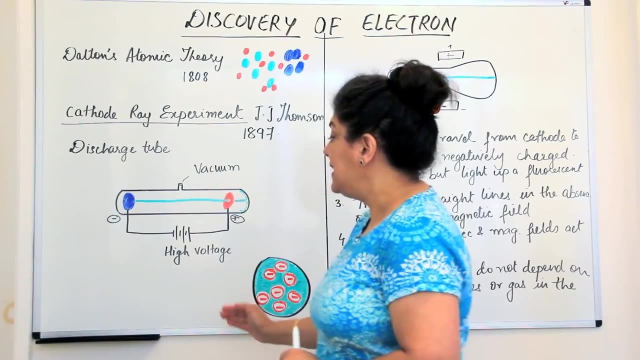 when he did that, he noticed nothing happened. so what did he do? he now reduced the pressure of the gas and he brought it down to 0.01, that is, he brought it down to a down a hundred times of atmospheric pressure and he increased the voltage of current to about a thousand volts and he found 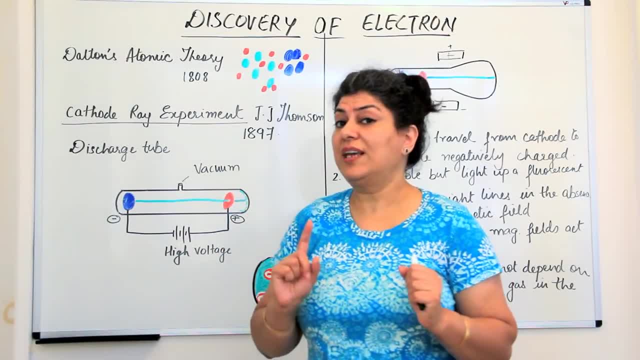 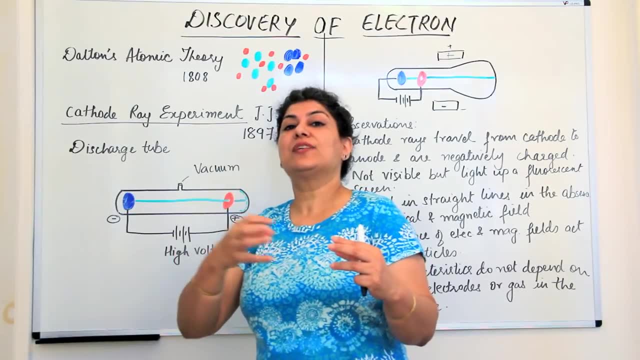 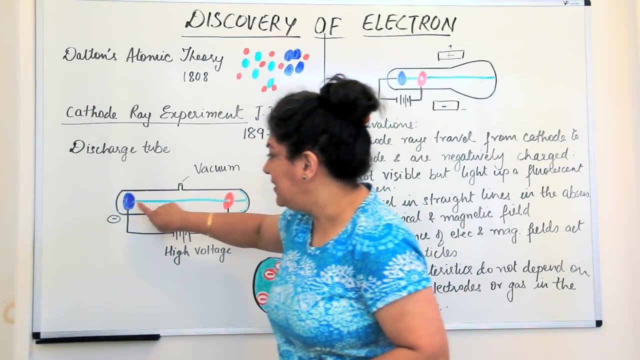 again that nothing happened. so he did not give up. he now increased the voltage to about 10,000 volts and he brought down the pressure of the gas to point zero, zero, one atmospheric pressure. now what did he notice? that there was a beam of light or there was something which was being given out a beam from. 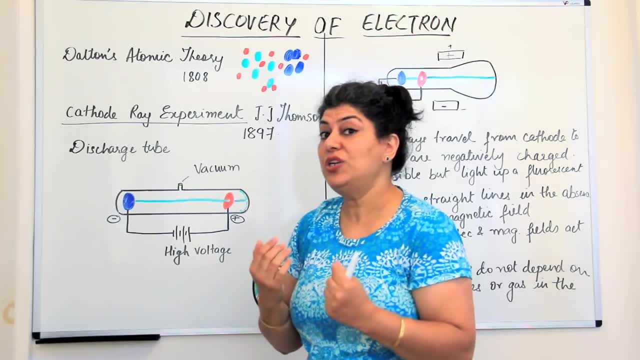 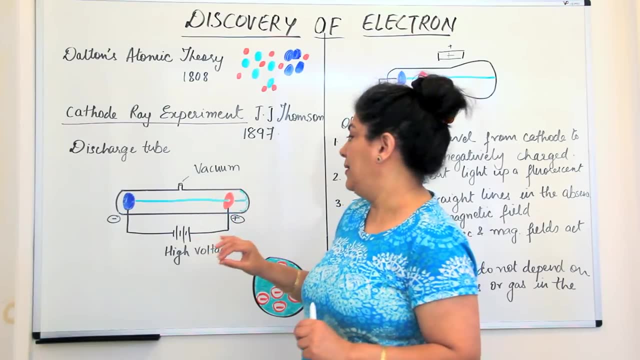 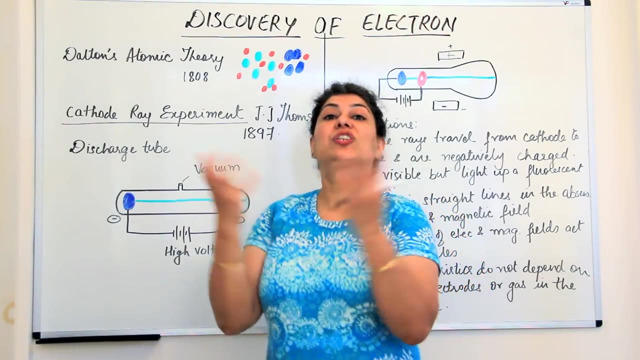 the cathode and it was moving towards the anode. and how did he learn about it? he could not see this beam, but behind the anode, perhaps there is a hole in the anode. he found that behind the anode, the screen which was coated with a fluorescent material. it got. 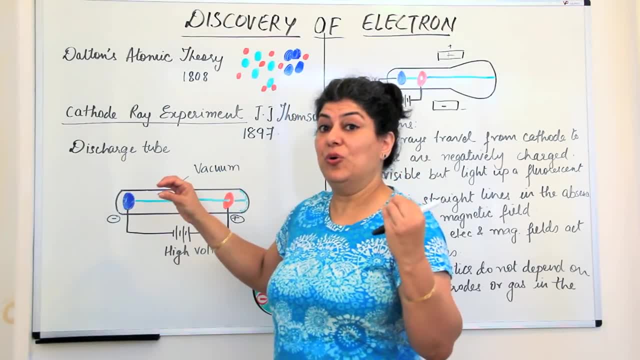 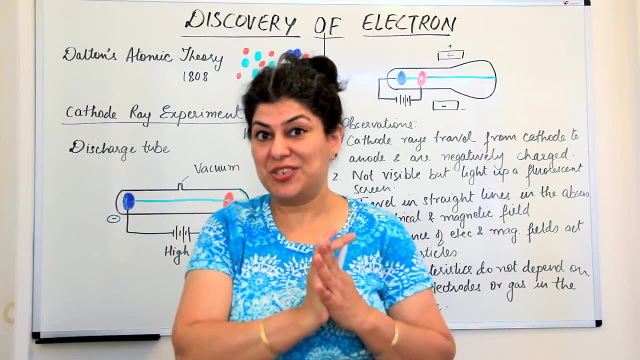 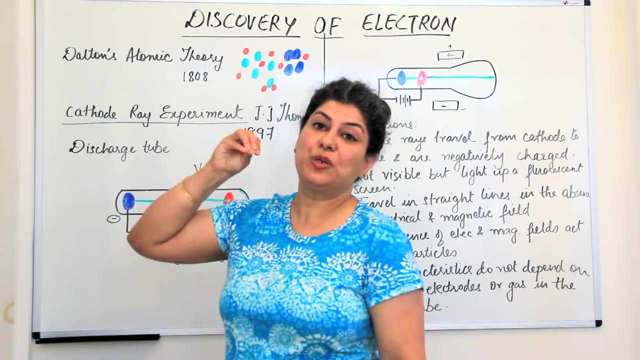 illuminated. this was if you know that it is the cathode ray tube, which is present in your television screens, which produces the images on your television screens too. even today, the television screen is coated with a fluorescent material and cathode ray tubes. it is those which give out the beams and the 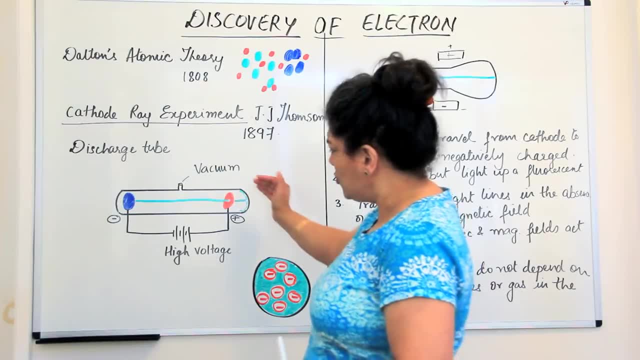 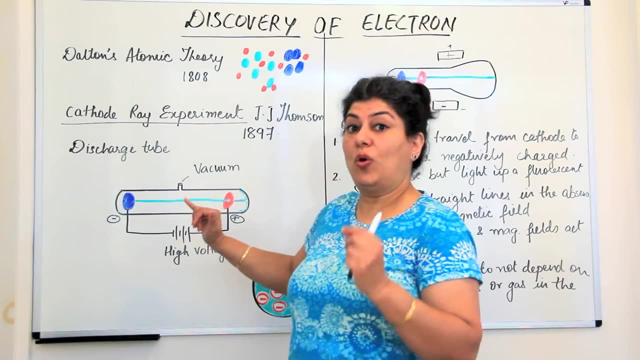 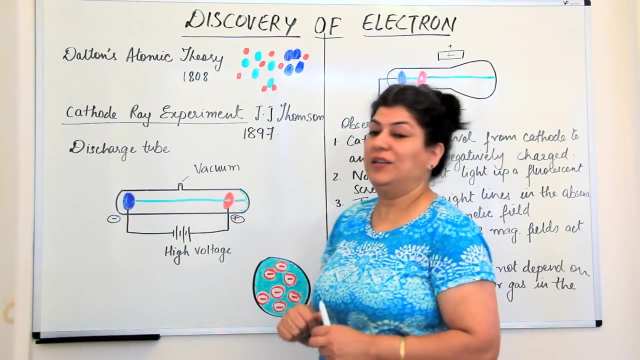 they get to illuminated and you see your images. so the same thing happened and he noticed that there was a, there was an illumination behind the anode. obviously, if the illumination was behind the anode, the ray must be coming from the cathode, so he called this the cathode ray. now what did he do? he wanted to know about. 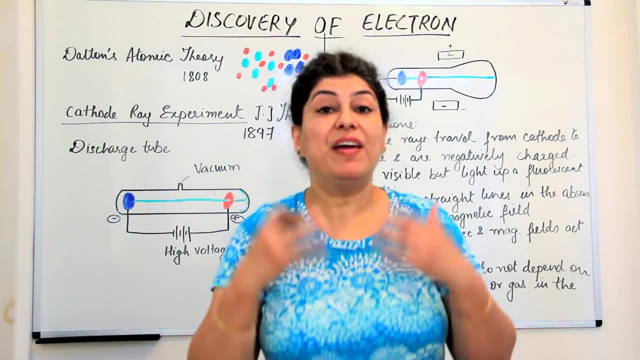 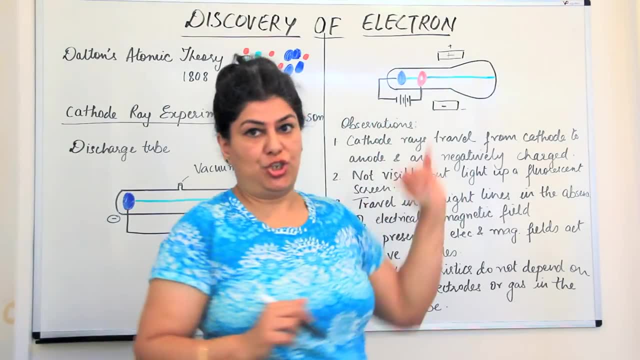 the properties of this cathode ray. what was it, where was it coming from and what was the source of it? what was the source of the solute and how was it coming from? the source of the solute, its nature. So what did he do? He took another discharge tube, and this time the discharge tube. 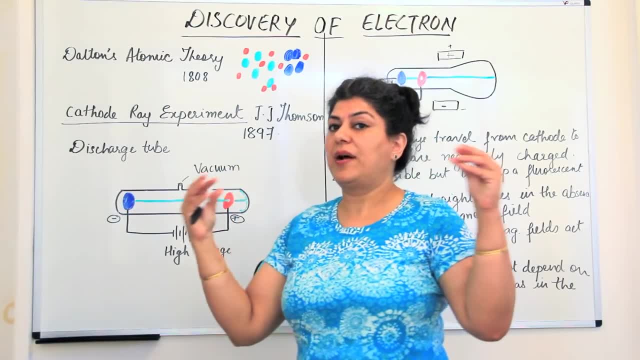 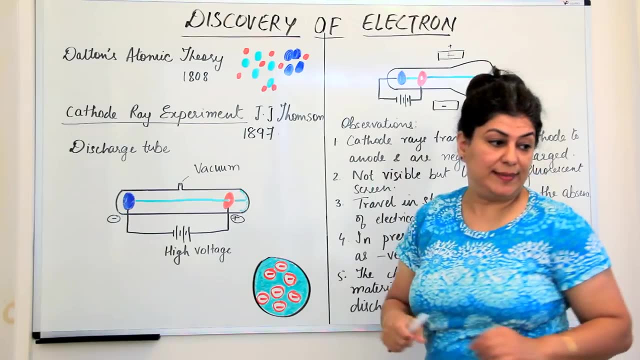 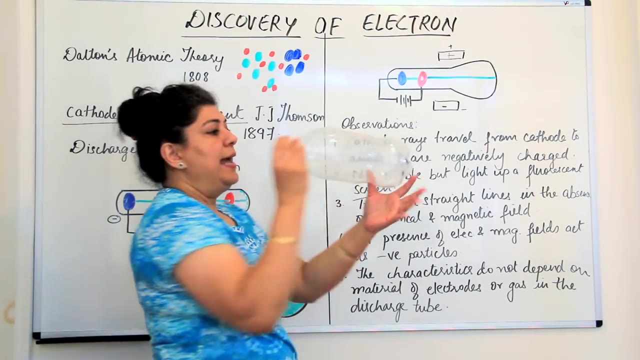 was not where the metallic discs were around the ends. He wanted to know about this ring, So he took a discharge tube which was somewhat like this: You can imagine this to be somewhat like a soda bottle. Do you see this Like a soda bottle? and if you imagine this soda bottle, he had these. 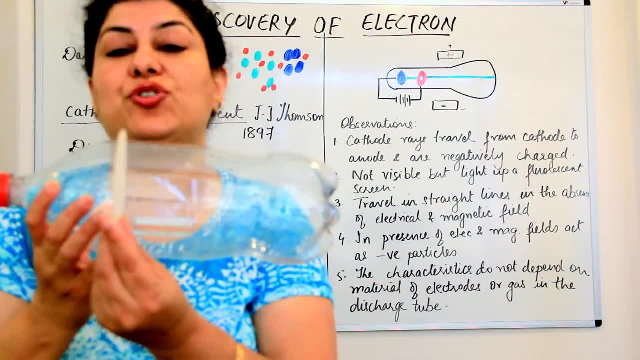 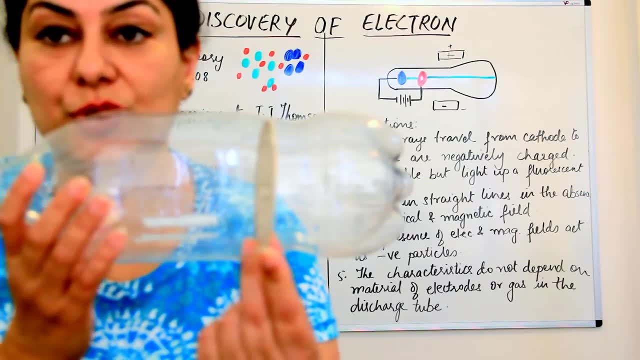 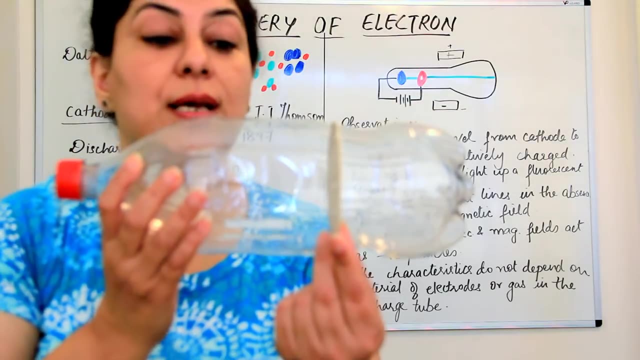 metallic discs which were, which were the electrode. So he had one disc here which acted as the cathode and one disc here which acted as the anode, A disc here and a disc here which acted as the cathode and anode, and the anode had a hole in it. So now, when he did this, what did he do When he passed? 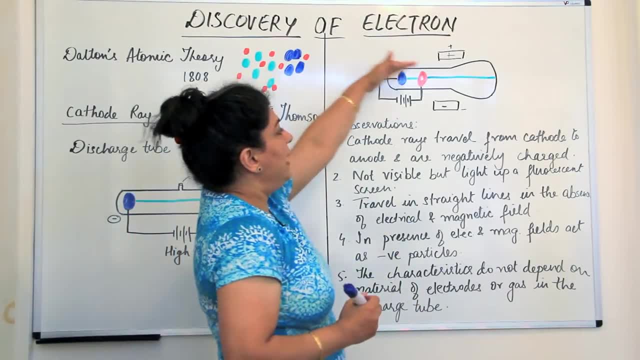 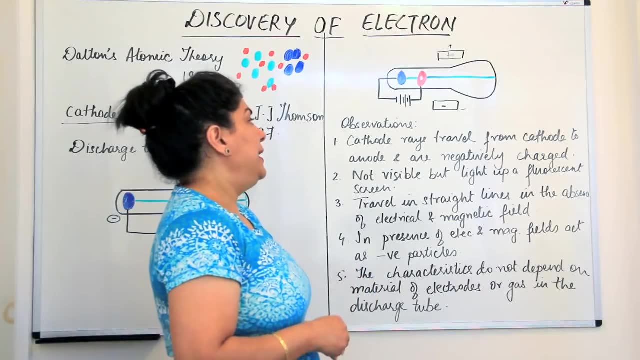 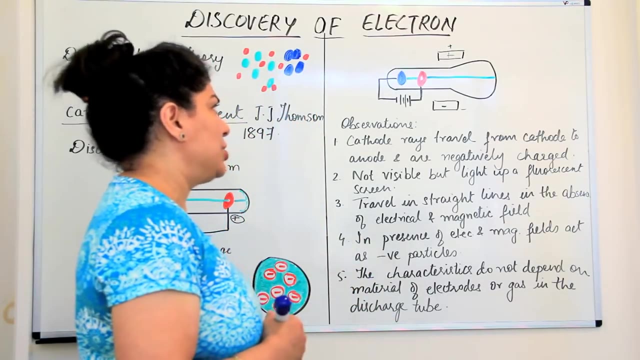 the electric current through it, that is, 10,000 volts, and the pressure was very low. he noticed that the cathode ray was produced and it was traveling in a straight line. He said that whatever this ray is, it is being produced by the cathode. Now he wanted to know its nature. He wanted to know: do all substances? 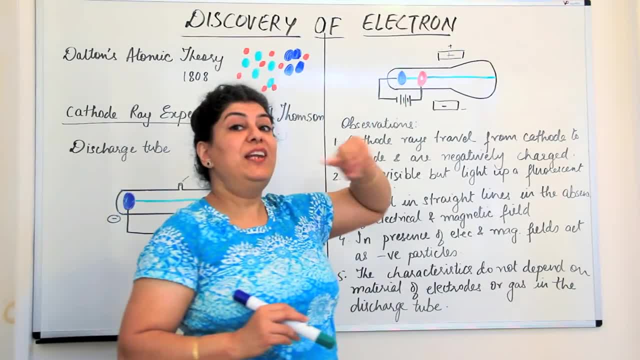 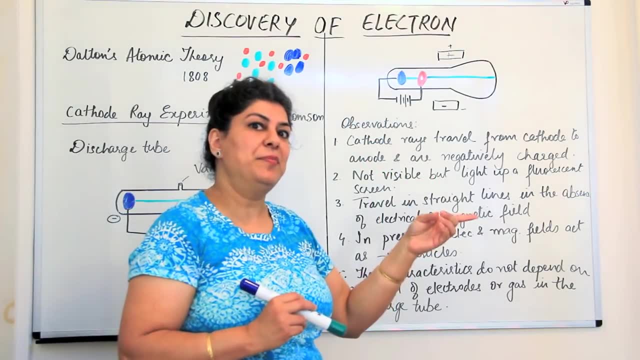 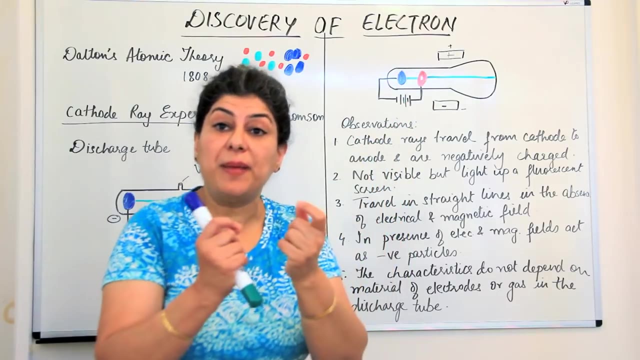 produce the cathode ray. So what did he do? He changed the gas inside the tube, the discharge tube. When he changed the gas, he still got the same ray. Then he swapped the metal of the two electrodes. Then he passed the electric current and he found he still found the cathode ray. 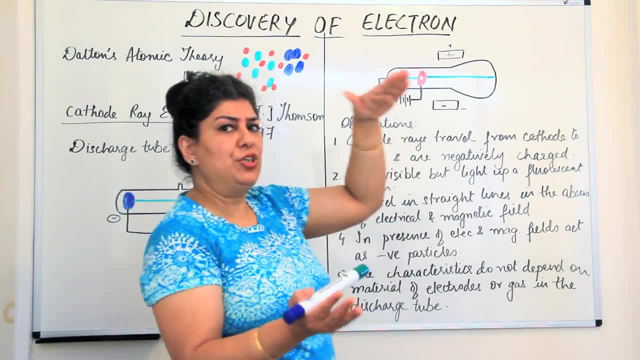 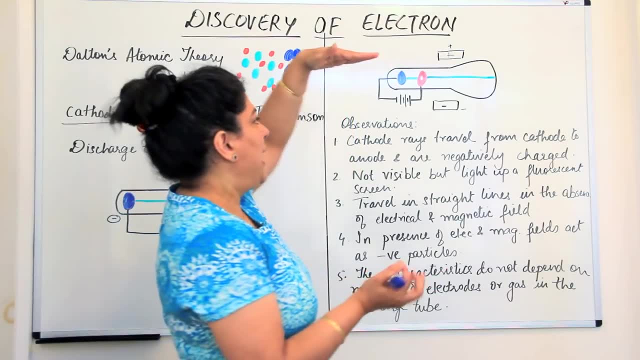 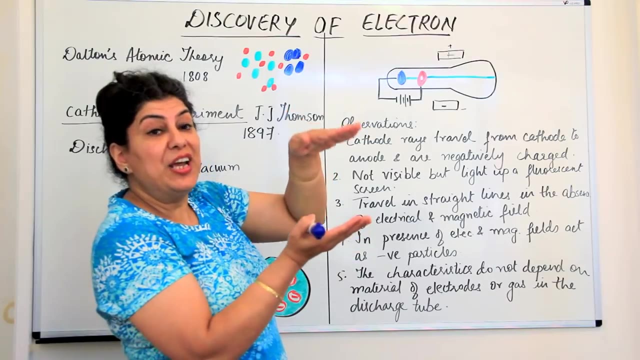 and now, what did he do To know the nature? he took two metallic plates, and these metallic plates were electrical plates. They were there were the two terminals, and he brought these two metallic plates above and below the discharge tube. When he did that, he was subjecting the ray to an electric 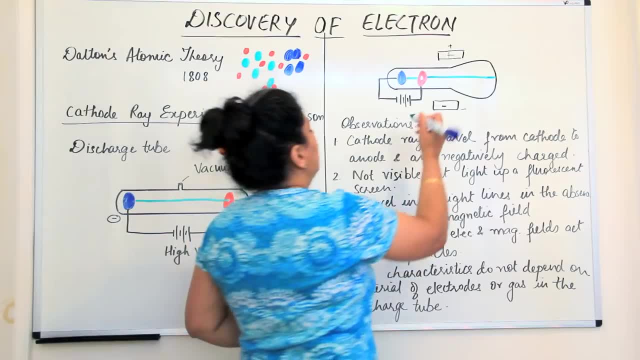 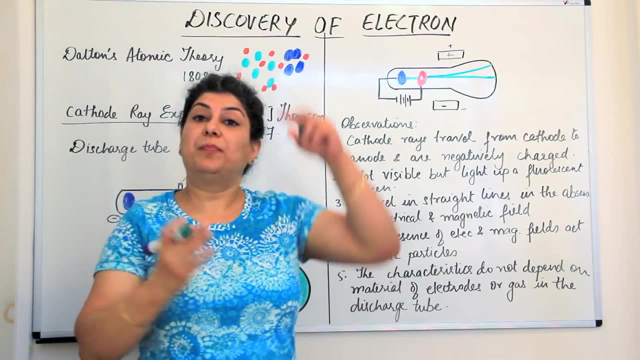 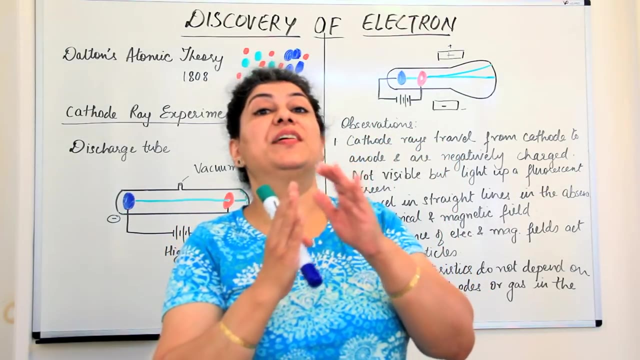 charge. and when he did that, what did he notice? He noticed that the cathode ray it deviated and itARSn y one, Mukysheut, bent towards the positively charged plate. What did this indicate? It indicated, we know, that electrical charges, like charges, repel each other and opposite charges attract each other. Therefore, 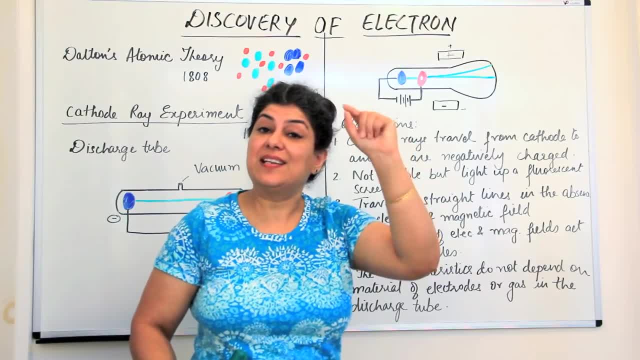 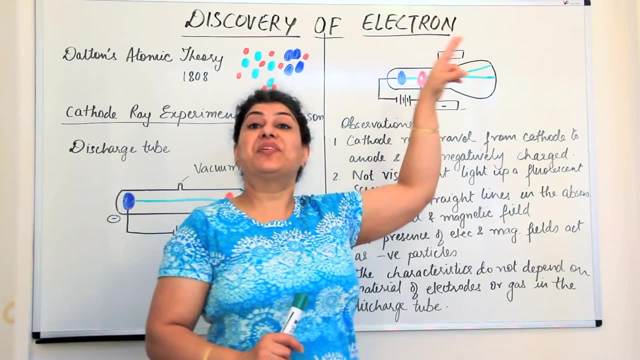 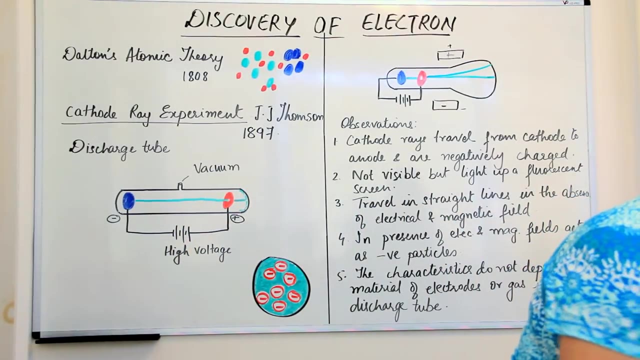 he concluded from this that cathode rays, they consist of particles which should be negatively charged. Why? Because it was moving towards the positive electrical charge, But he still wanted to make sure. So what did he do now? He took a- let us say that this was the discharge tube- and he 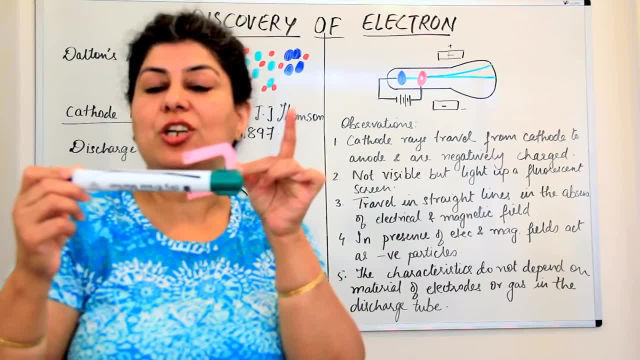 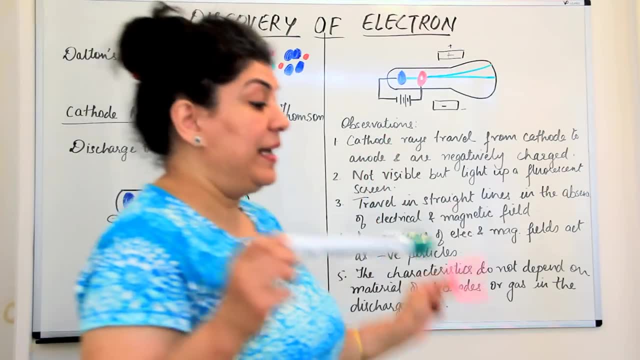 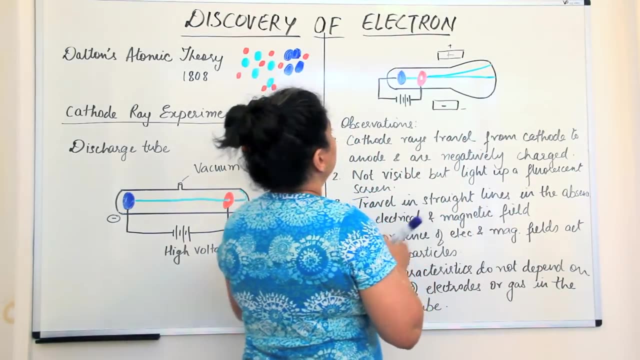 took a magnet and this time he subjected the discharge tube to a magnetic field. and when he subjected it to a magnetic field and not the electric field, what did he notice? this time, When he subjected it to a magnetic field, he again noticed that the cathode rays they moved towards. 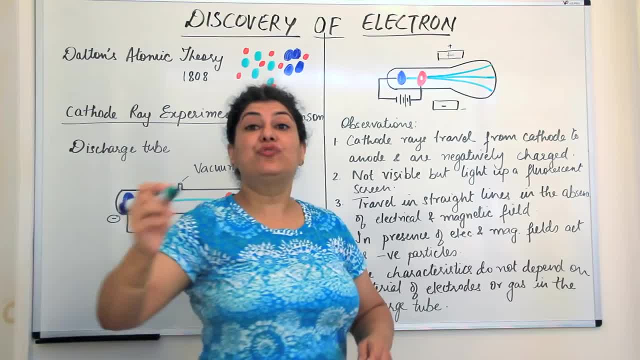 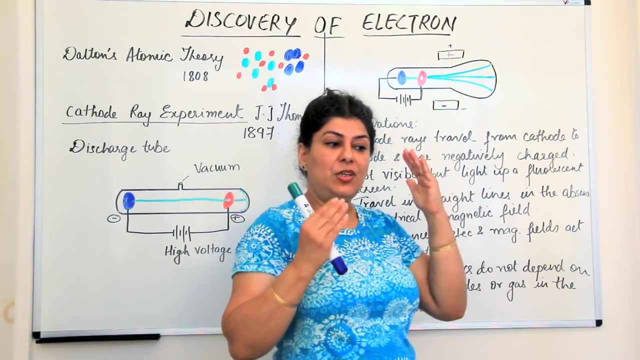 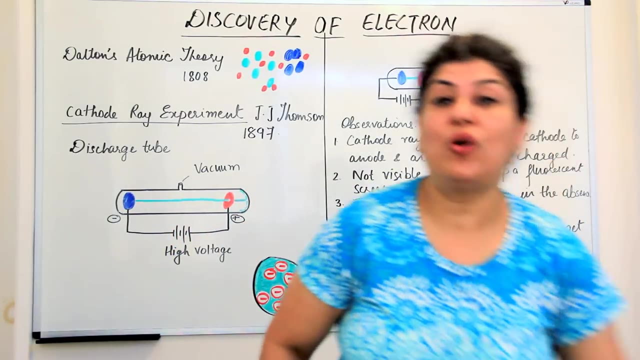 the other direction And they moved in that direction, which would be expected or if of any ray which is negatively charged. So the behavior that the cathode ray was showing in the presence of electrical and magnetic fields was those of negatively charged substances or negatively charged particles. So 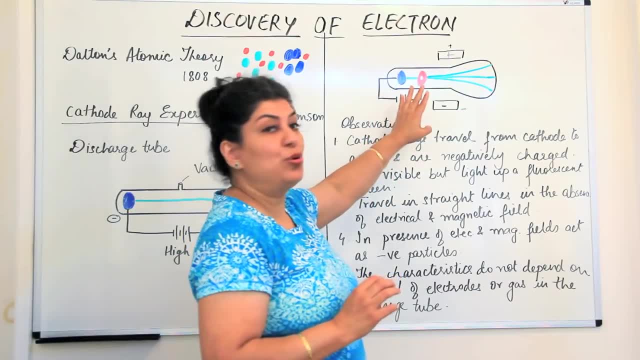 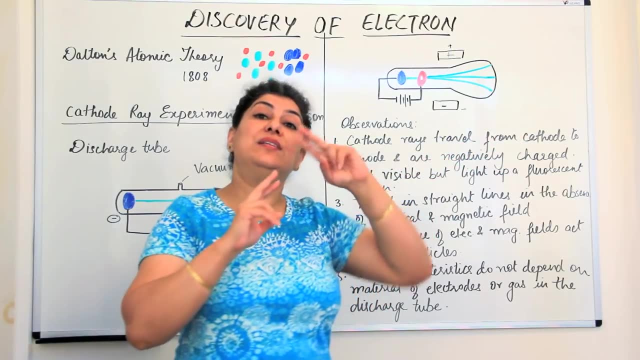 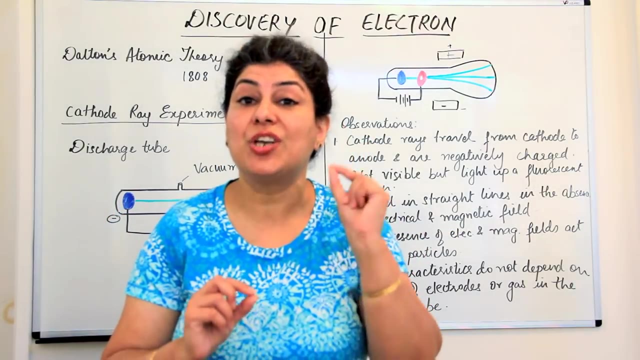 and since he swapped the metal of the cathode ray tube, he said that whatever be the substance, we still got the same Same ray from different electrodes, from different gases. therefore, all matter should consist of this negatively charged particle. Then, through some other experiments, he found out that the mass of 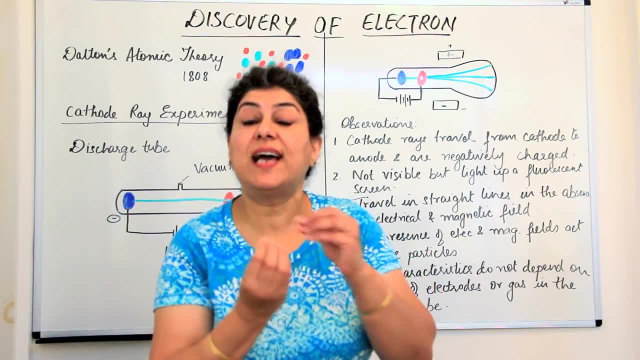 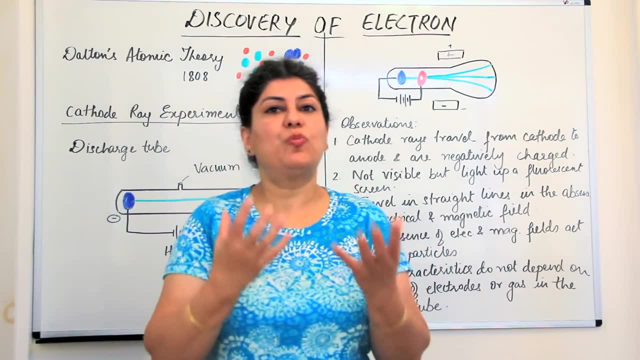 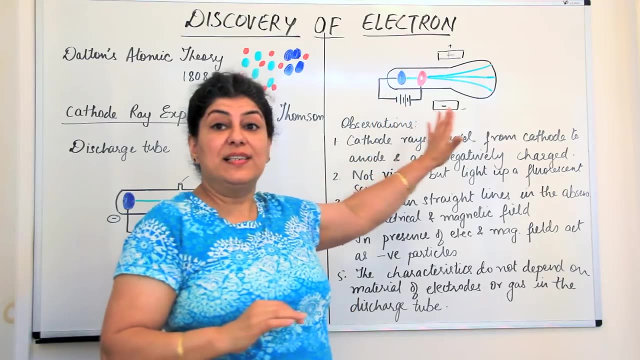 this particle is a thousand times less than the mass of hydrogen, But by now scientists felt that hydrogen was the smallest atom and there could be nothing smaller than an atom. That's what Dalton had said. But this revealed that an atom consisted of something which was smaller than an atom, and even hydrogen, since. 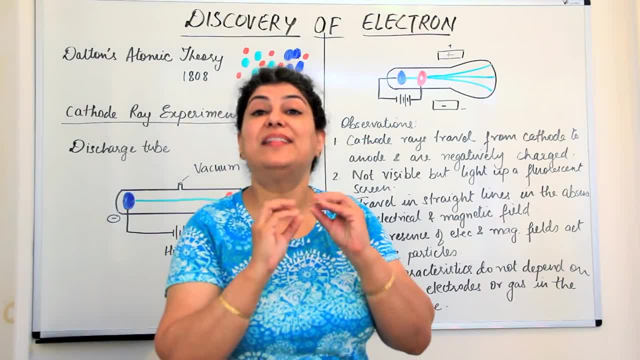 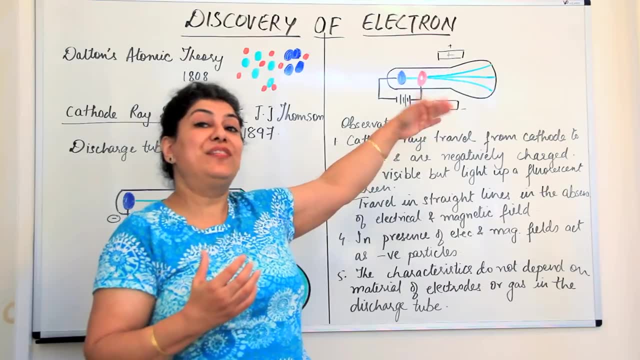 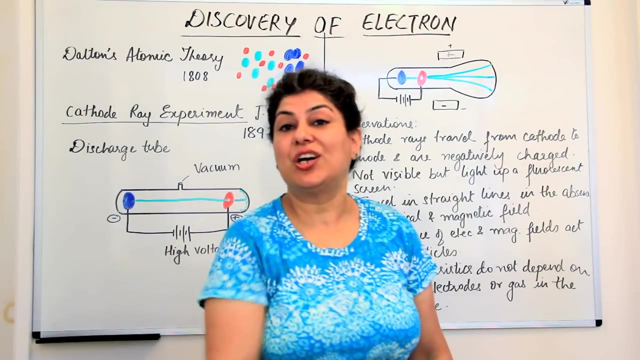 he took hydrogen, there was something which was smaller than the hydrogen. obviously it would have been given out by the atoms, So he said. and since, on switching the different elements, he found the same results. he said all atoms of different elements consist of a negatively charged particle. 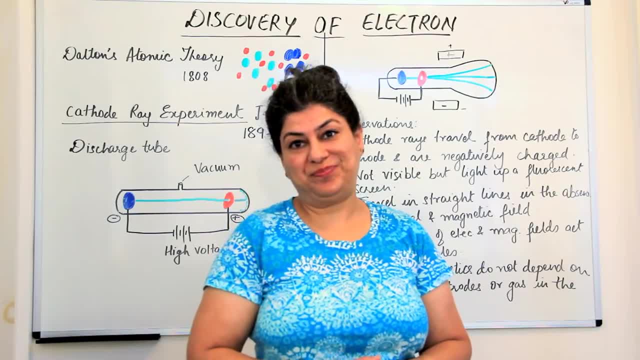 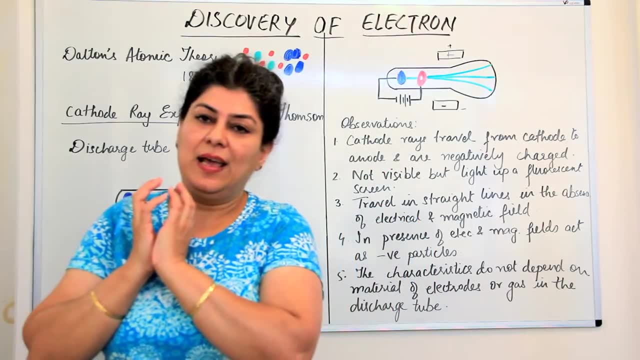 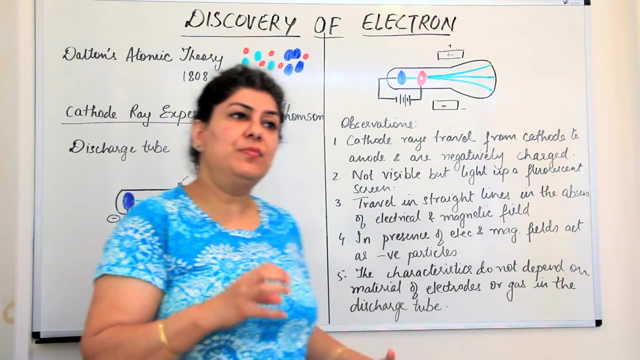 and he called this particle the electron. But this is not the case. This is not the case. But then he said: if an atom consists of electrons, then what should an atom look like? On the whole, he knew, an atom is neutral. and since, on the whole, an atom is neutral, the atom he imagined.